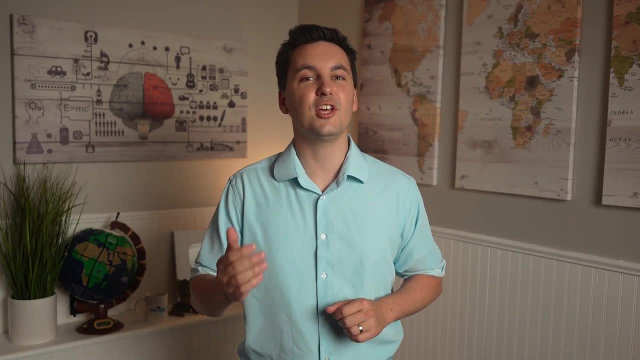 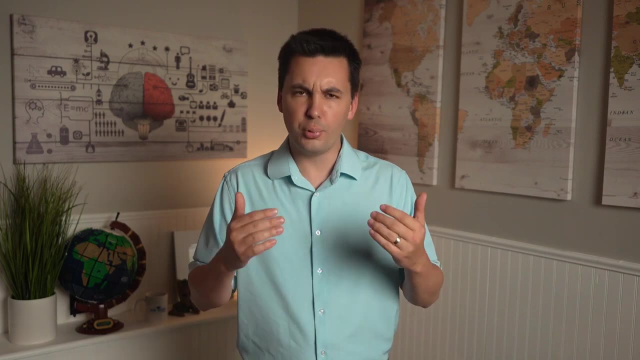 people into a place. If we look at societal factors, we can see that societies that discriminate against different ethnicities, genders, sexual orientation, races or religions create push factors that motivate people to leave an area, Areas that also lack healthcare services. 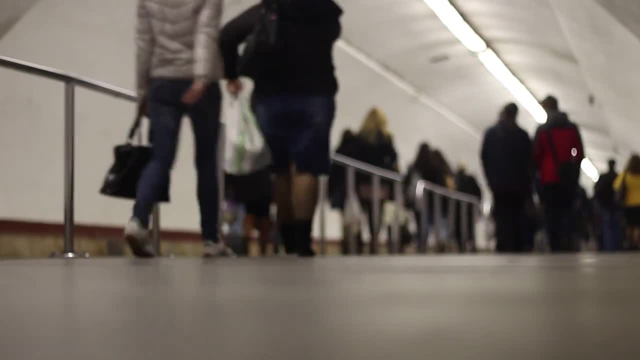 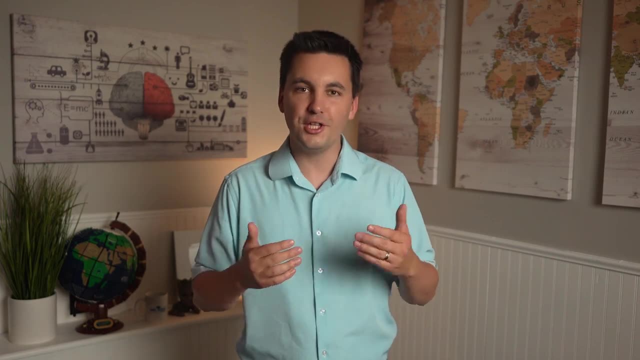 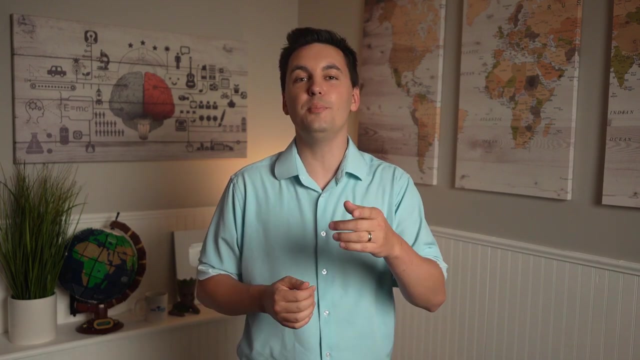 have poor educational systems or lack public services will also push people out of the area, Whereas places that offer religious freedom, are accepting of all people, offer quality education and healthcare services and have less income and gender inequality will see more pull factors as people will be drawn. 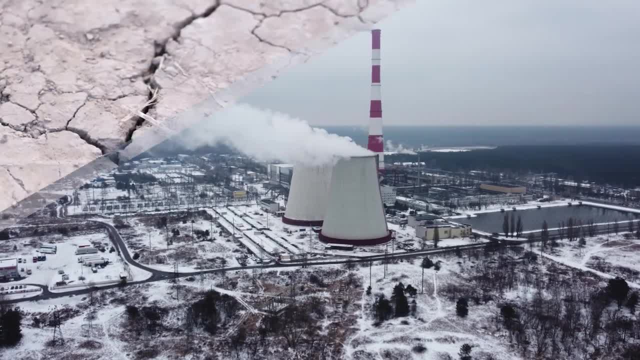 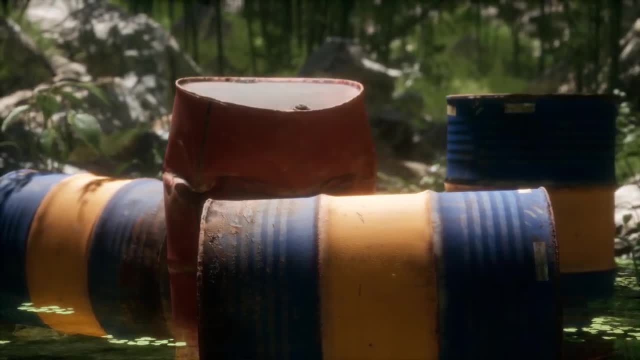 to that area. Then there are environmental factors. Places that lack arable land, water, have a higher chance of having a natural disaster or human disaster, such as a chemical spill or pollution from factories often will push people out of the area, But societies that 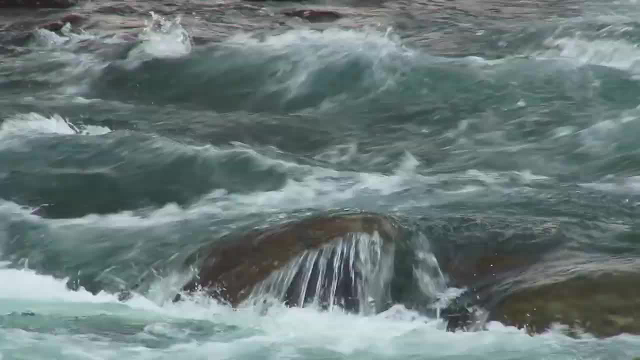 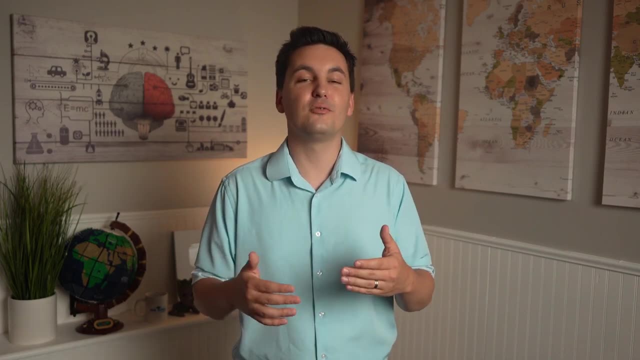 are located in areas that have arable land, clean drinking water and preferred climates will motivate people to move to those areas. One thing to remember when it comes to push and pull factors, especially environmental ones, is that some factors will differ depending on who 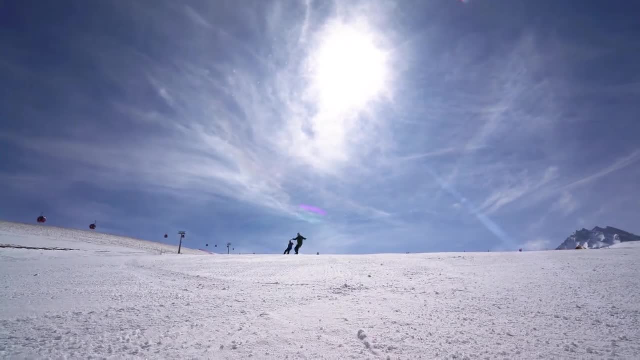 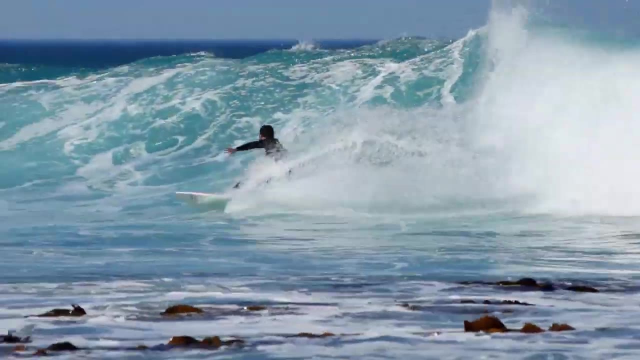 you talk to. For example, a person who likes to snowboard may consider a place where it's more cold and snows more often more appealing than a place where it's always sunny and warm. But someone else, for example a surfer, will most likely consider the cold a push factor and would rather 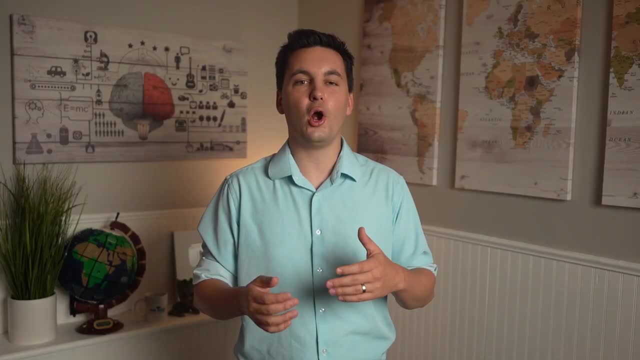 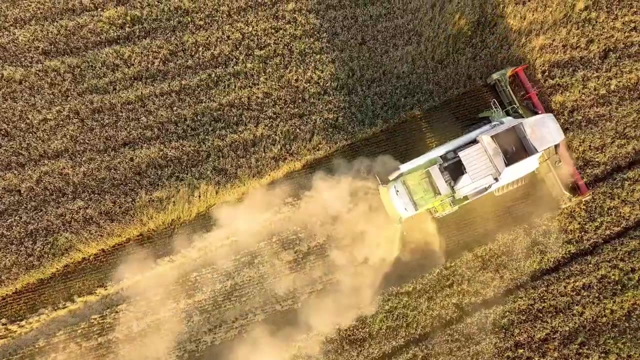 live near a beach with air or water, For example, if you're living in a country that has a lot of access to the ocean, Or a business that needs a large workforce will most likely see a large urban area as a pull factor, But a business that requires lots of land and a smaller workforce. 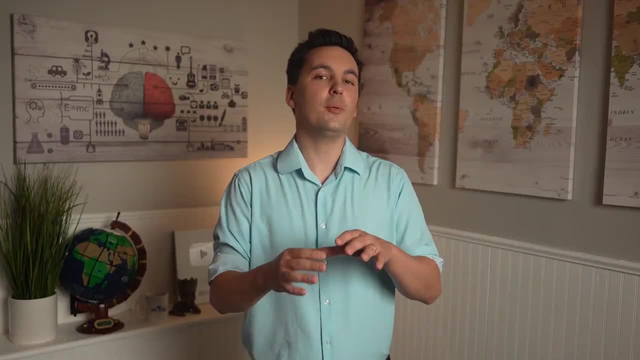 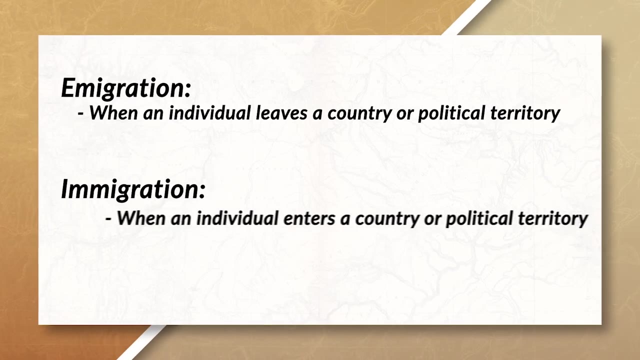 will look for more of a dispersed population with cheaper land. Now, going back to migration, we can see: if a person is leaving a place, it's known as emigration, And if a person is moving into a place, it's known as immigration. For example, I currently live in the United 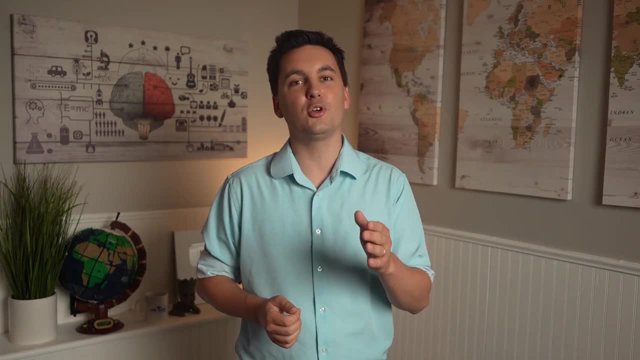 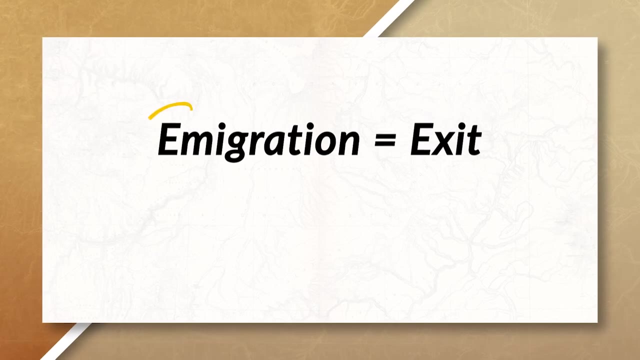 States of America. But if I decide to move to Australia, I would be emigrating from the United States and immigrating to Australia. To make sure you don't mix these terms up, think of emigration as E for exit and immigration as I for in, So we can see that people migrate.